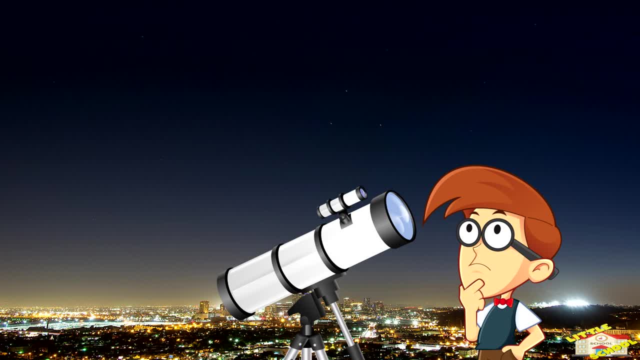 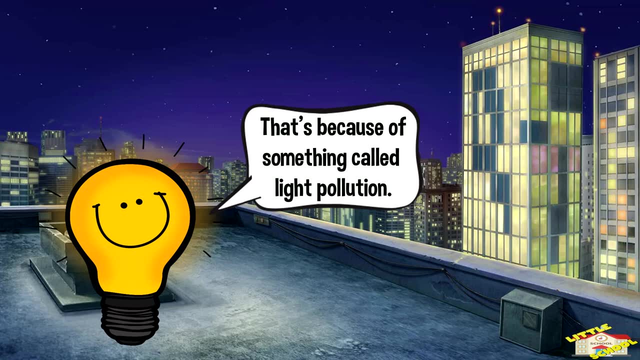 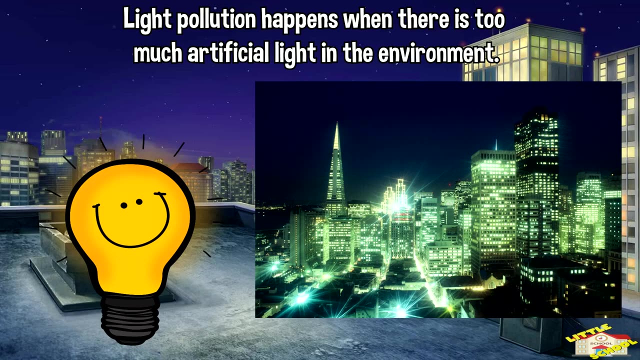 you might not be able to see as many stars as you would in a darker area. That's because of something called light pollution. Light pollution happens when there is too much artificial light in the environment, especially at night. This excess light makes it difficult to see objects in the sky such as stars. 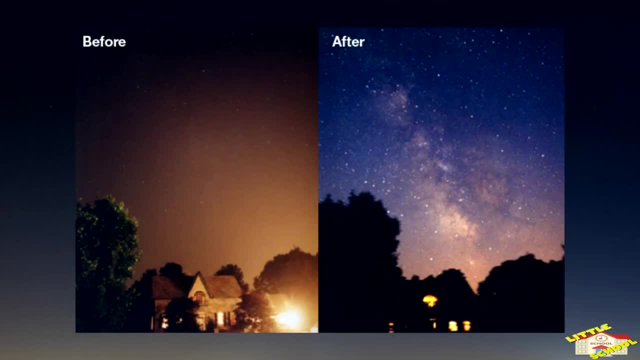 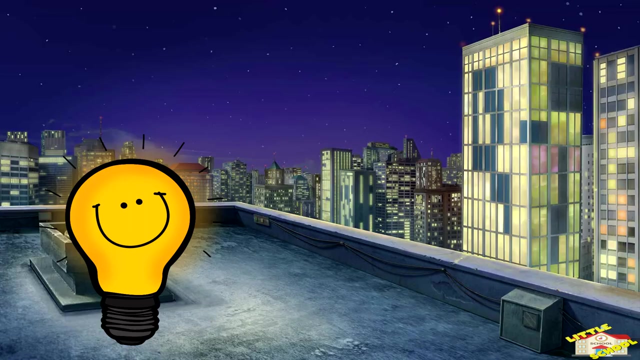 To the left, it shows us how much light pollution affects how we see stars in the night sky. On the right, it shows us that with no light pollution we can see the stars clearly. There are a few types of light pollution in the night sky. 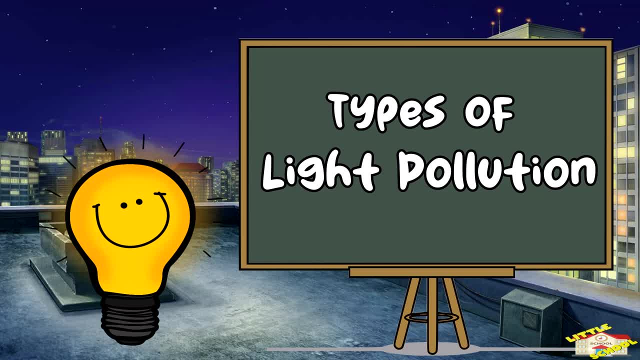 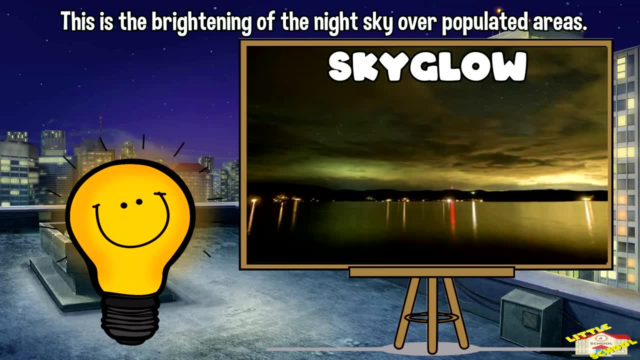 One of them is light pollution. There are a few types of light pollution. Sky glow. This is the brightening of the night sky over populated areas. Instead of seeing a dark sky full of stars, the sky looks kind of hazy and illuminated due to scattered light. 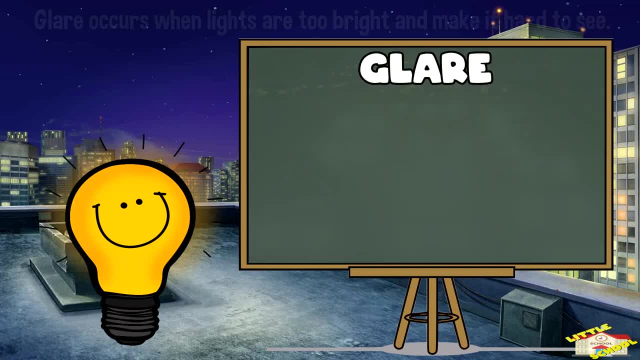 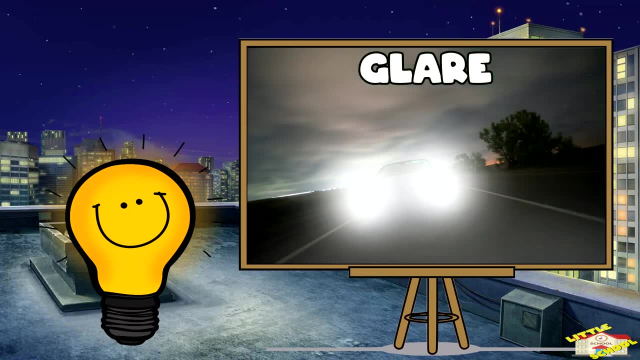 Glare. Glare occurs when lights are too bright and make it hard to see. For example, if you're driving at night and someone has their headlights on high beam, it can be blinding. This is a form of glare and it's a type of light pollution. 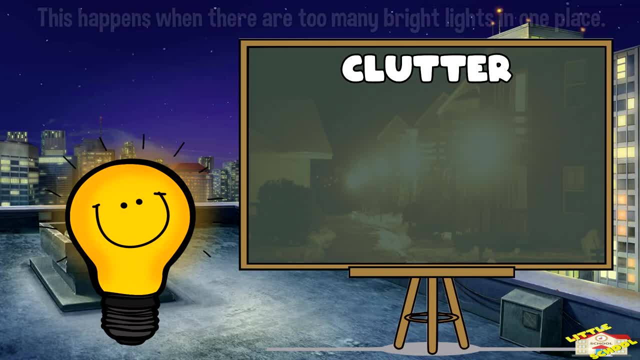 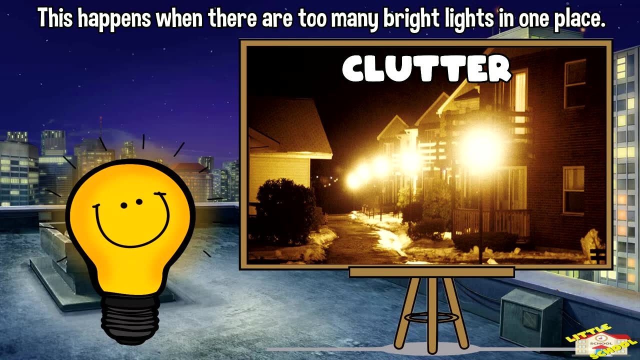 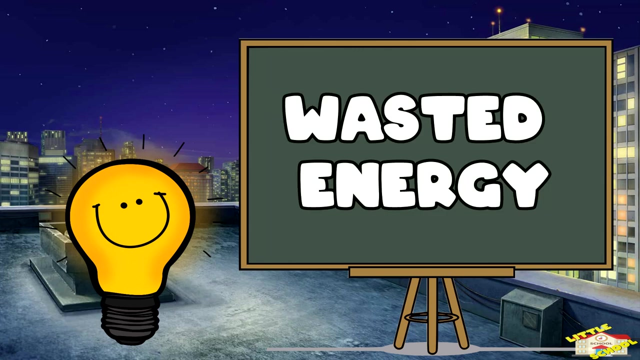 Clutter. This happens when there are too many bright lights in one place, making it challenging to focus on specific objects or details. It can be distracting and make it harder to see things clearly. What are the negative effects of light pollution? Wasted energy. 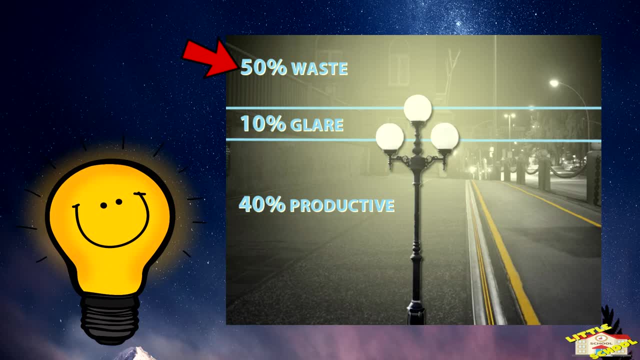 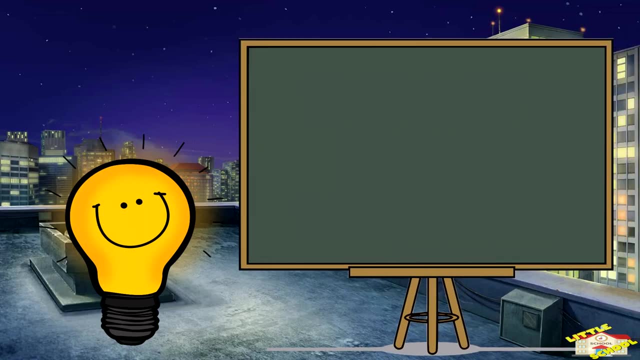 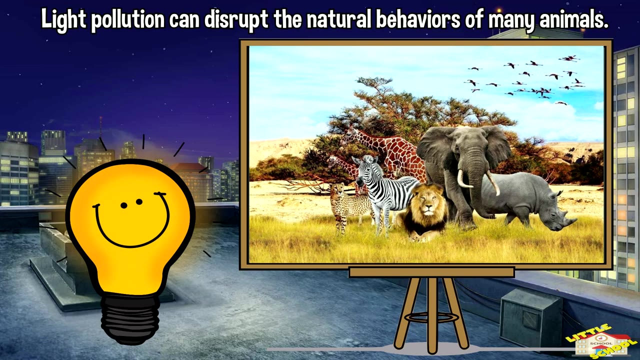 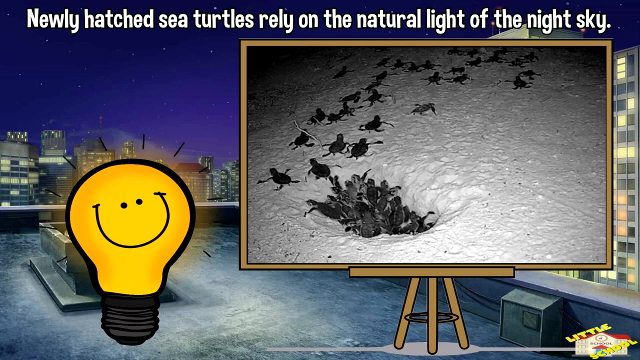 A significant amount of the light used for outdoor lighting is wasted by being directed where it's not needed. Impact on wildlife: Light pollution can disrupt the natural behaviors of many animals, Including birds, insects and sea turtles. For example, newly hatched sea turtles rely on the natural light of the night sky to find their way to the ocean.